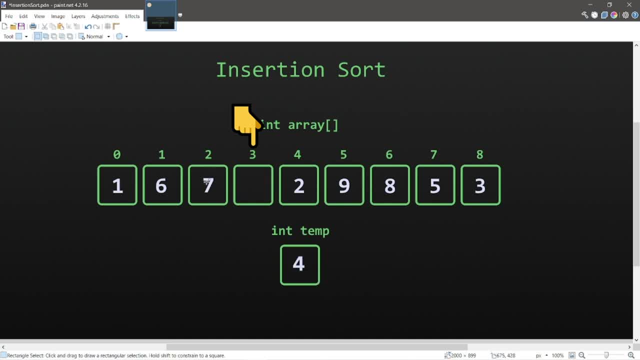 place it within temp. examine the elements to the left. If they're greater than four, we shift them to the right. Seven is larger than four, shift it to the right. Six is larger than four, shift it to the right. One is not larger than four. so we stop here. take whatever is within temp, this value. 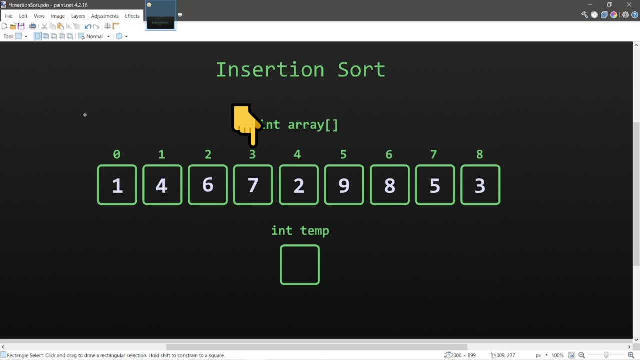 four and insert it here into this opening. So that was the first three iterations. We repeat this process until we run out of elements, So I'll speed up the footage. So we are currently on index four. Thank you, And that is your visual representation of the insertion sort algorithm. I like to think of it. 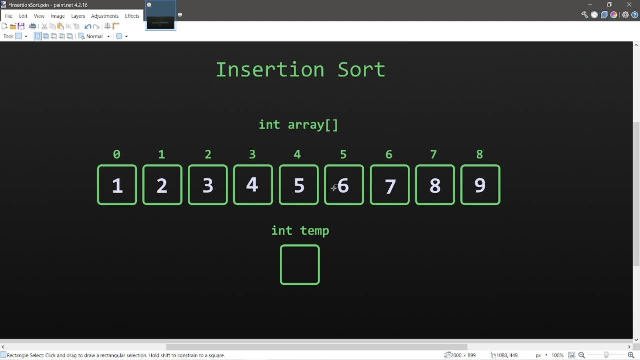 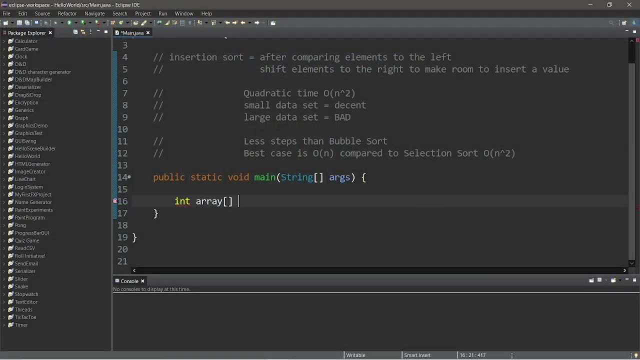 like a jigsaw puzzle. We have some pieces that are connected, they fit together, and we will move whole sections of pieces together to make room for a piece that fits. So let's create our own insertion sort algorithm in JavaScript. We'll need to create an array. Let's create an array of integers, int array and make up some. 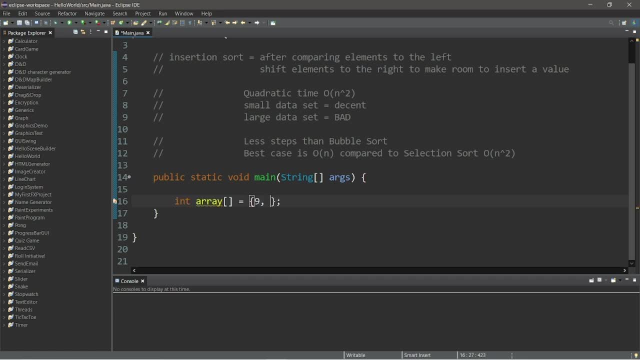 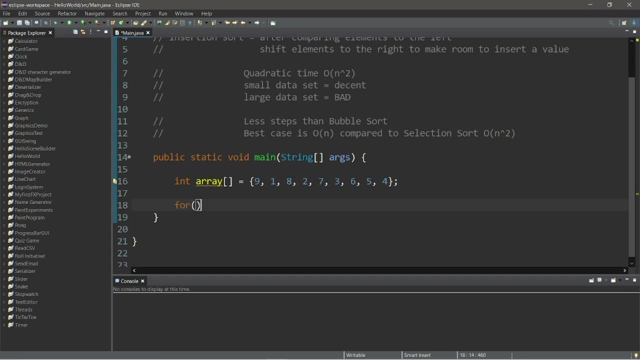 numbers. Put whatever numbers you want within here, Maybe nine, how about a one and an eight and a two and a seven, three, six, five, four. That sounds good to me. Okay, then let's display the elements of this array. We'll use a for each loop, For int i in array. we will display: 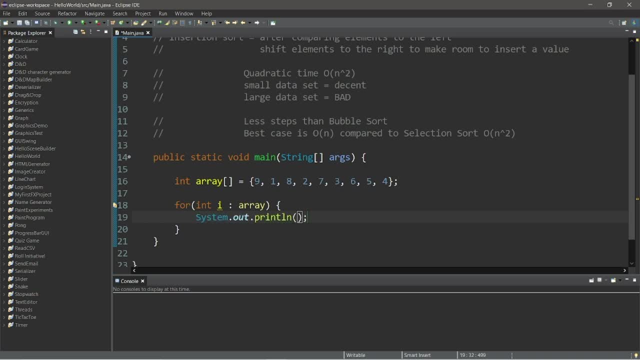 each element within this array with a print statement. So let me get rid of that print ln and just have print. So I will print i. I think I'm going to add a space afterwards. I didn't do that in the previous two videos, so I think I better do that. Okay, let's just run this just to test it. 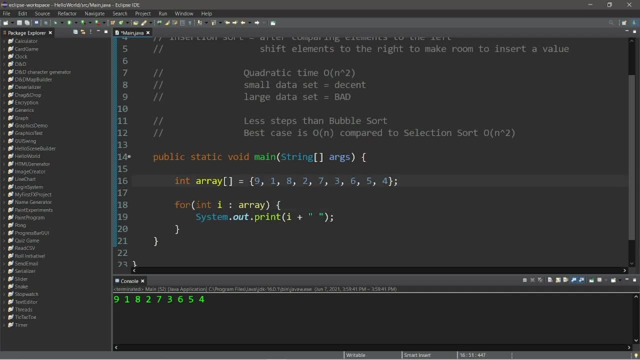 Nine, one, eight, two, seven, three, six, five, four. And before we display the elements of our array, let's invoke a function which we still need to declare, called insertion sort. So insertion sort. Then we will pass in our array as an argument and we'll need to declare this: 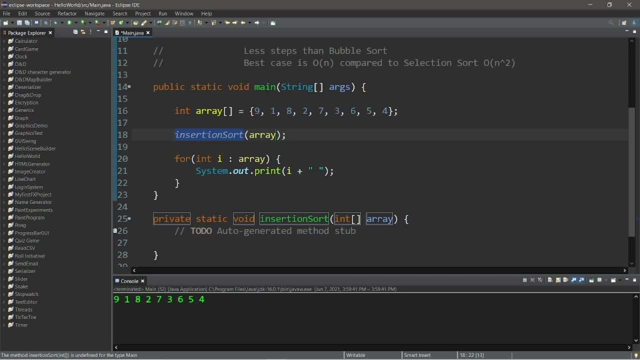 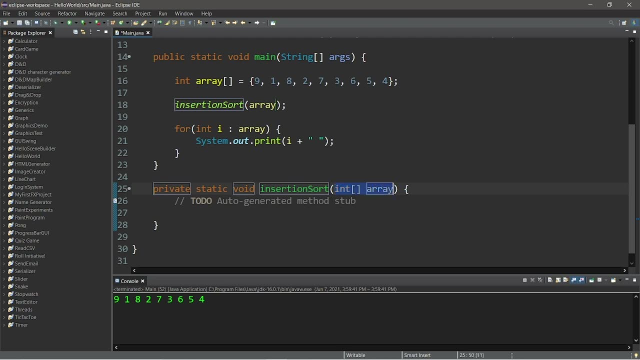 So I'm going to cheat and create this automatically. So, outside of our main method, create a method named insertion sort- Private static void insertion sort. There is one parameter and array of integers. Okay, now the first thing we'll do is create a for loop to iterate over. 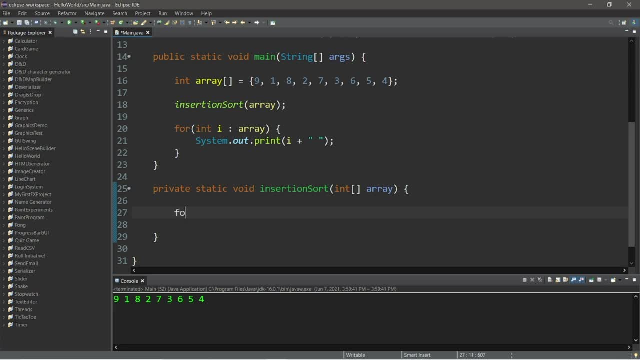 each element of our array, but it begins at one, not zero. So that would be four, And we will set int i to equal one, not zero. Pay attention to that. We will continue this as long as i is less than array dot length And we will increment i by one during each iteration. 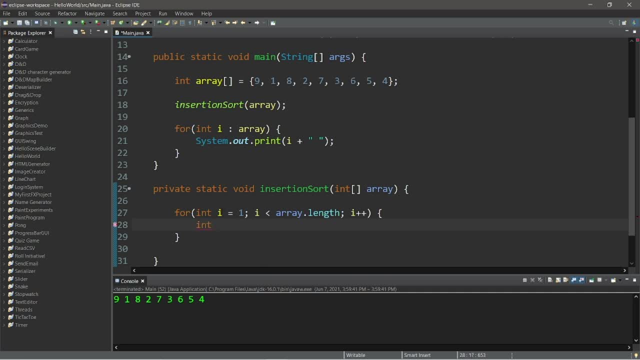 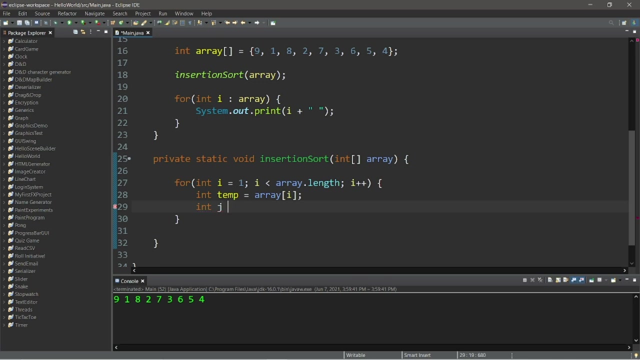 Now we need to take our value found within i and place it within temp. So let's declare a temporary variable named temp Int. temp equals array at index of i. And now we'll create a variable named j Int. j equals i minus one, So this will keep track of. 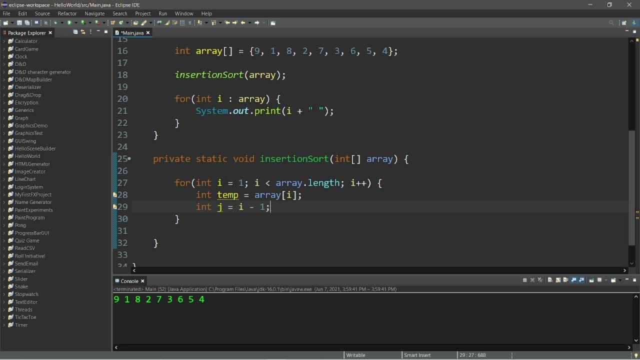 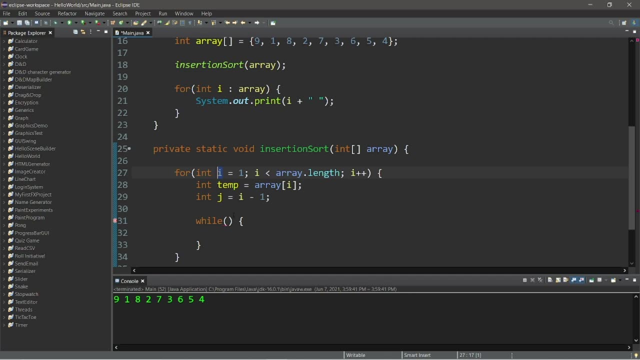 what value we're comparing to the left of whatever i is. So, then, we need to create a while loop. We will continue comparing values to the left of i, And our condition is going to be: while j is greater than or equal to zero and 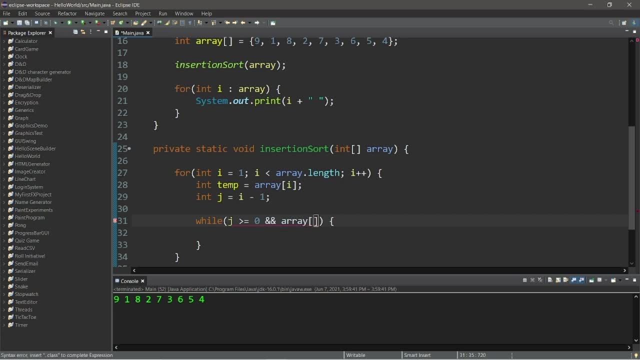 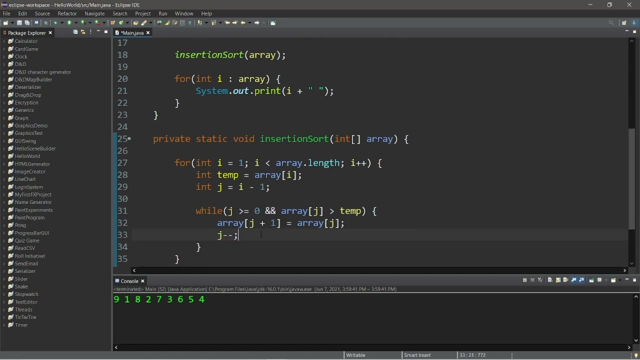 around. So if we need to shift an element to the right, we would say array at index of j plus one equals array at index of j. So that will shift an element to the right. Then we will decrement j by one, j minus minus.